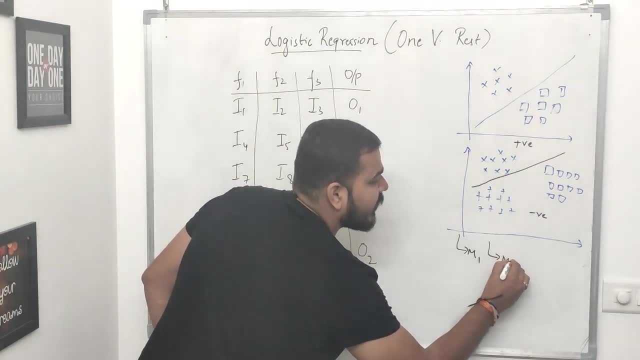 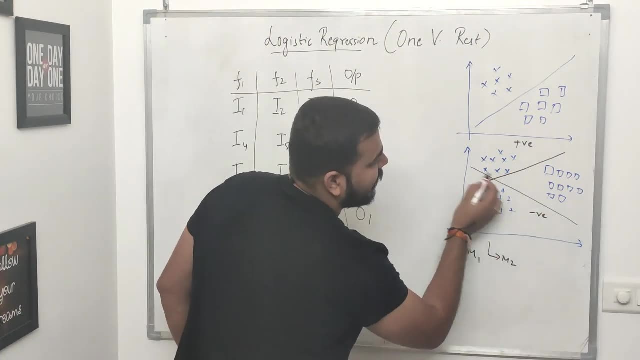 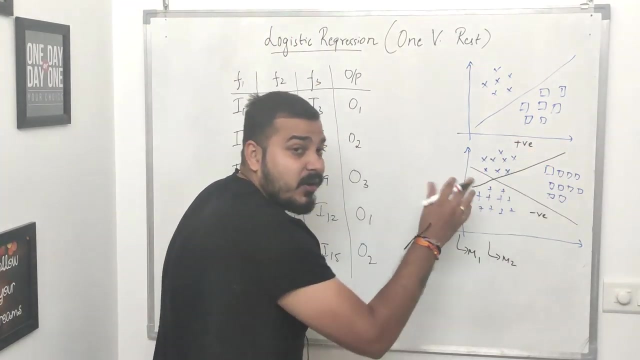 happen is that in the next thing is that another model, m2, is actually created. and now what it does is that, in the m2 category, first of all, it will consider this two categories as one- okay- and this separate category as a positive category- okay. in the second case now, based on the number of 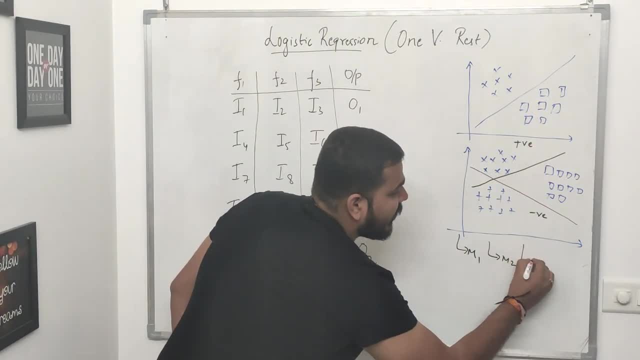 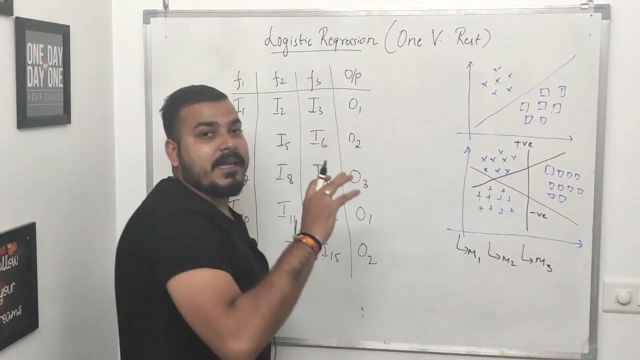 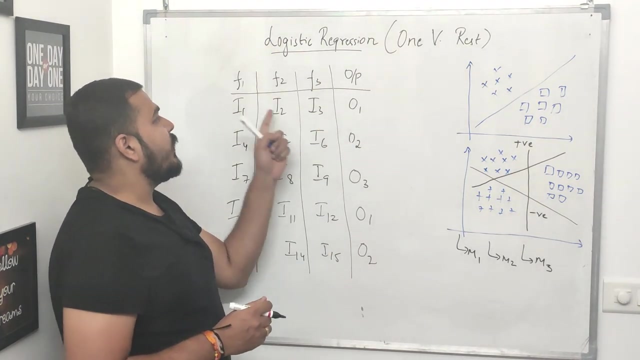 categories again, since there are total three categories. in the next iteration the model m3 will be created, wherein these two categories will be treated as one and this particular category will be treated as a separate positive category. so like this combination will be taken up. now, if i consider this particular example you can see over here: 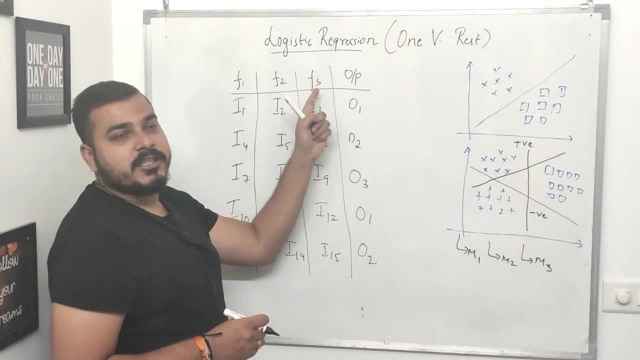 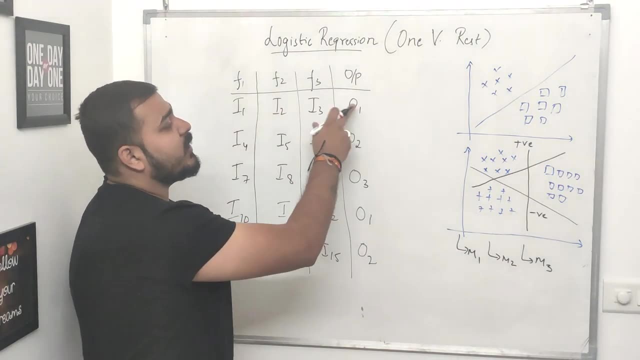 suppose i have feature f1, f2, f3. this is my independent feature. i have an output feature away as o1, o2, o3. so these are all my output features. based on the input i1, i2, i3, the output is got as o1. okay, similarly, if my input is i4, i5, i6, my output is o2. so like this, all the records. 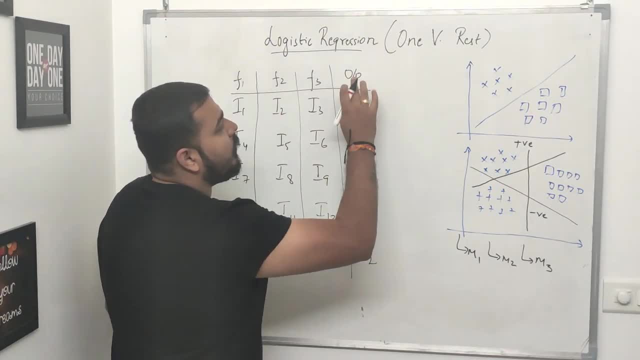 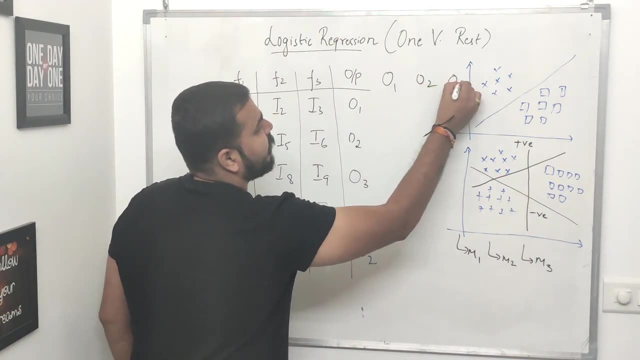 i have actually having away now how this all categories will get splitted. now, what will? what it will do is that now i have, suppose, three categories: o1, o2, o3. okay, now, considering this, what i told? i told you that whenever i have o1, that will be treated as plus one. okay, then i have 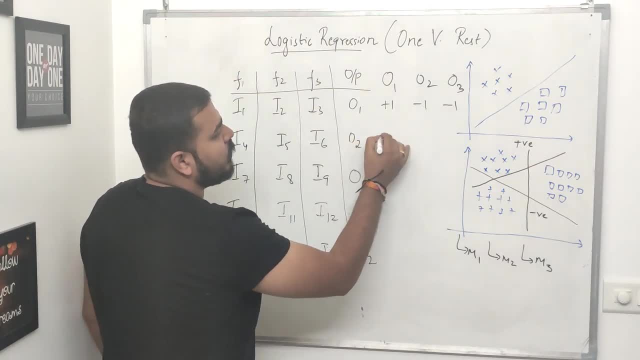 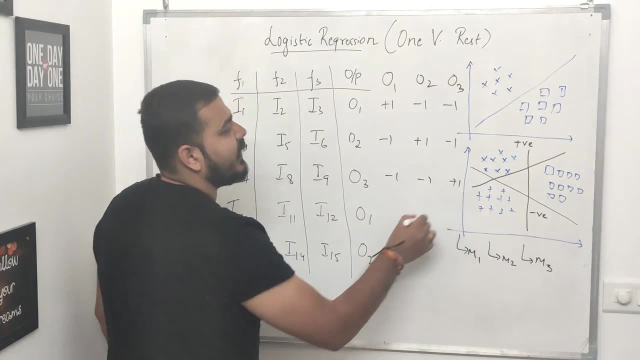 o2 and o3 will be treated as minus one. similarly for o2, in this particular case, this will be minus one. this will get treated as plus one, and again minus one. o3 minus 1, minus 1: this will be treated as plus one. so like this, all the combination will be taken up. now, here you have plus one. 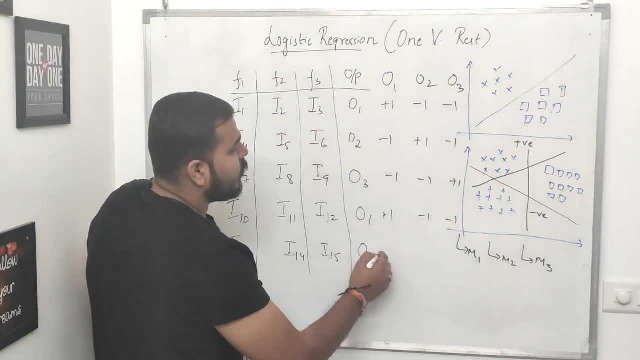 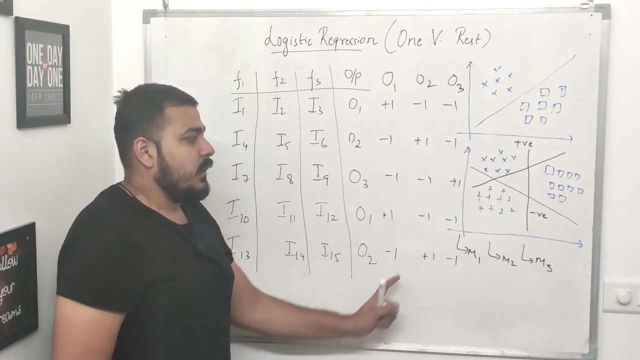 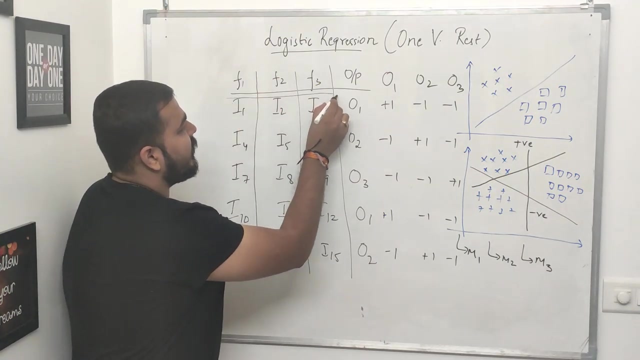 then again here you have minus 1, minus 1.. now, similarly, in o2, you have over here as minus 1, plus 1 and minus 1. now, considering this logistic regression, when we are using one versus rest, the first model that it will create it, they are going to take this independent features. 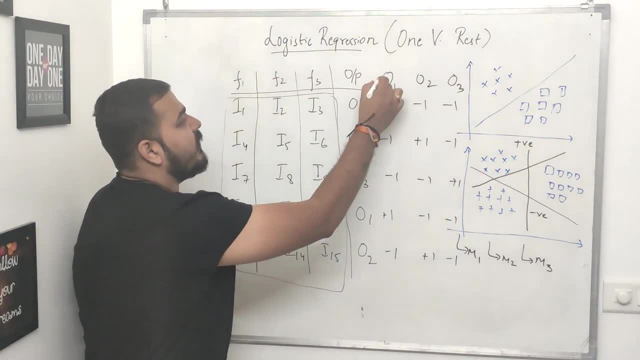 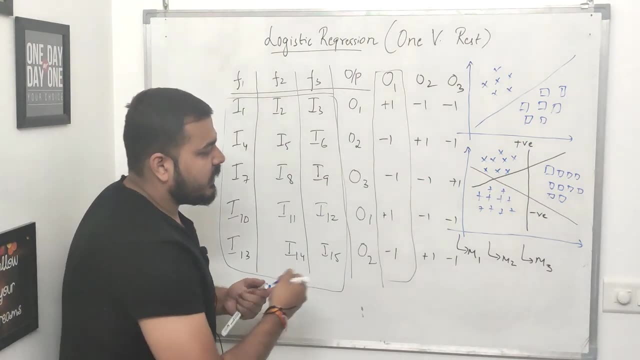 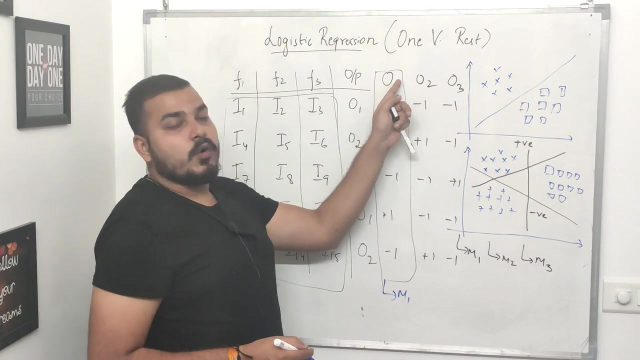 all the independent features. right apart from that, they will take this first output, one feature which will be my output feature, and based on this, based on this, they will create the model m1. okay, so the model m1 will be able to find out whether it is o1, whether o1 is positive or it. 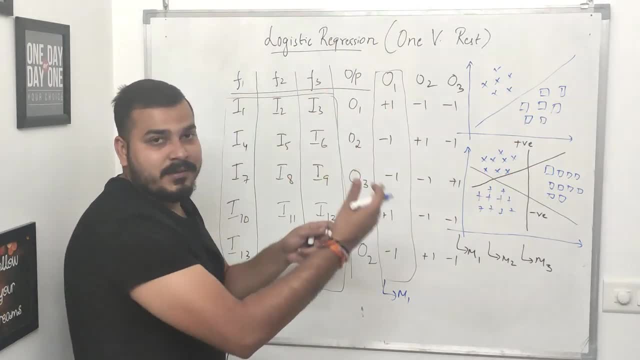 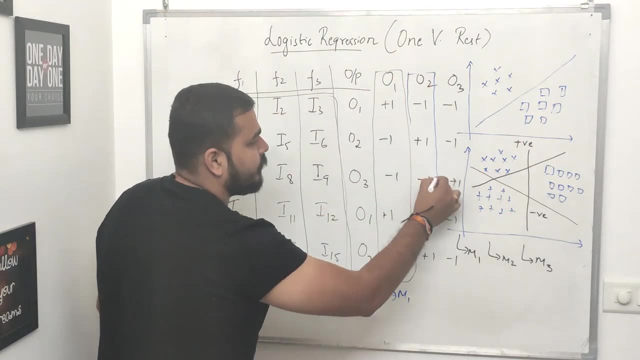 is negative or not. okay, now, similarly in the next model, that is what it is going to do- is that it is going to take this input feature and the output feature will be taken in this particular column. that is my o2, and for this again, the next model, m2, will get created. 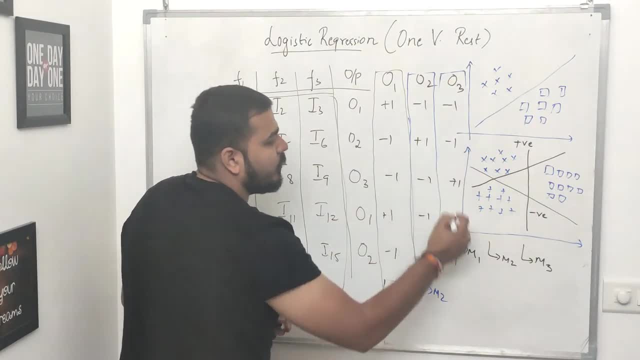 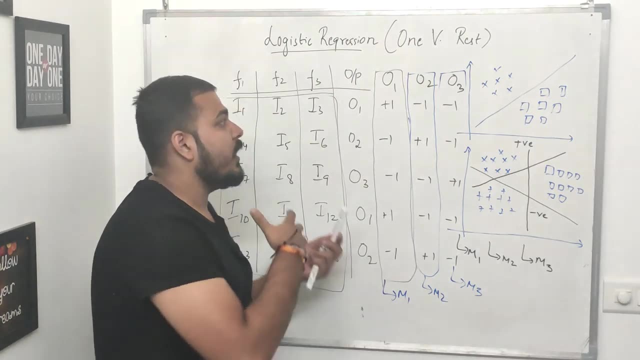 okay, and similarly for this particular data: final, my output. this will be my m3 model. now you may be considering that if i give a new test data, how will the model actually find out? how will the logistic regression find out the output? so, whenever i'm giving a new test data, 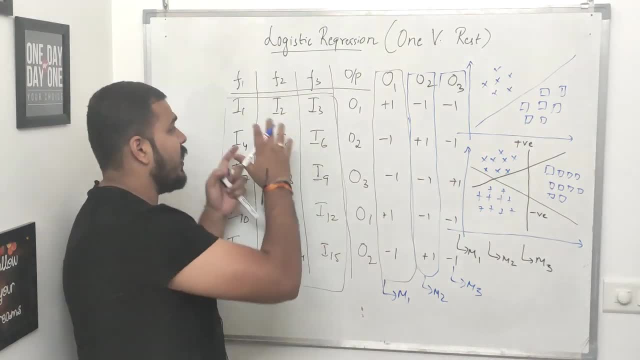 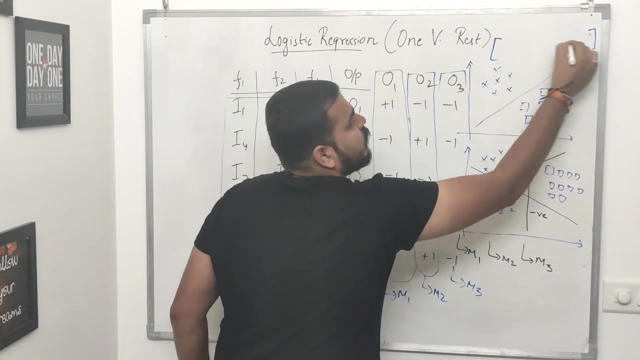 the this whole model, this m1, m2, m3 model. first of all, this whole input feature will go to the m1 model and when it goes to the n1 model it will give us one probability value. suppose this gives us 0.20. my m1 model gave me the answer as 0.20, which is my probability. 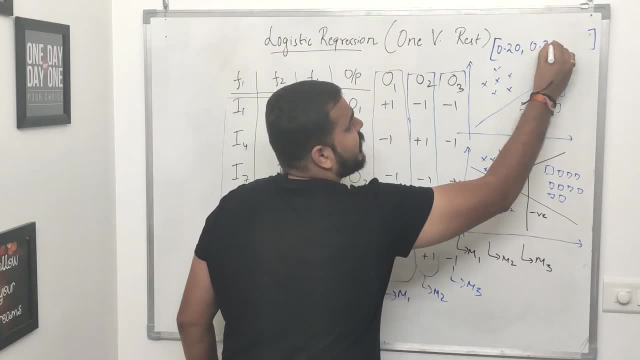 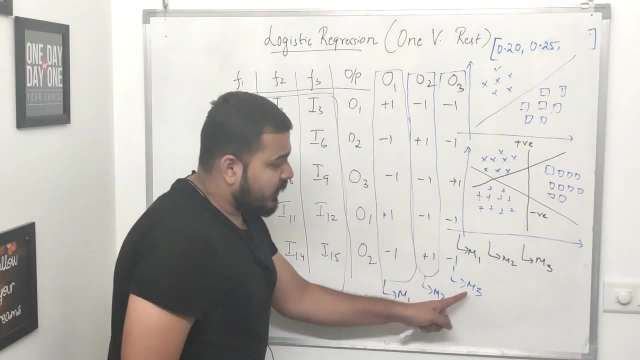 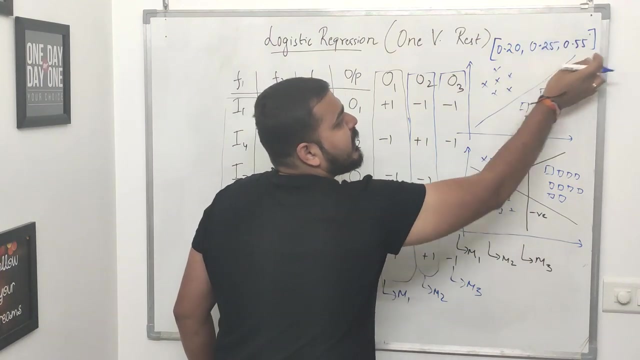 then my m2 model basically will give another probability like 0.30. okay, or i can say it as 0.25, suppose okay, 0.25. then the same data set will be given to the m3 model and suppose the output is somewhere over here as 0.55. now you can see the sum of all this. 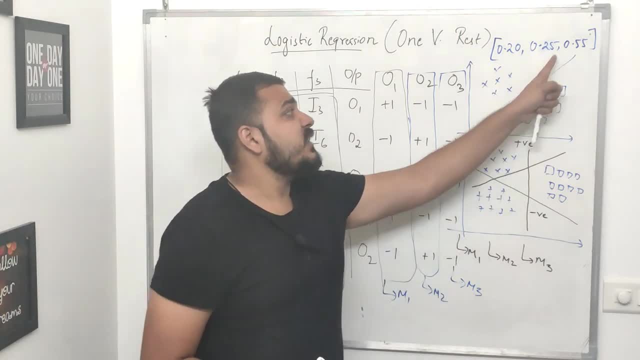 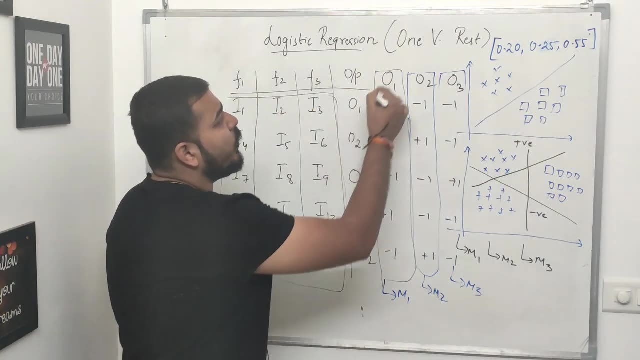 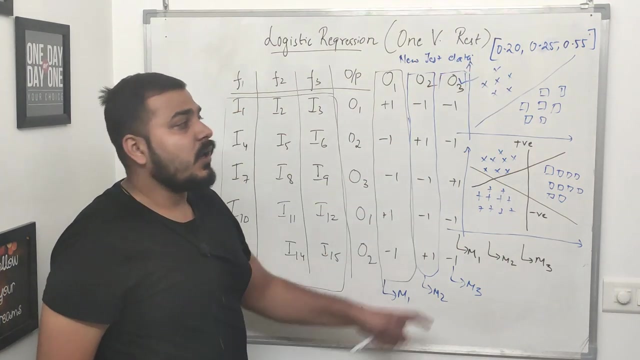 thing is actually one. okay, then it will go and check which is giving the highest probability. suppose my m3 model is giving the highest probability of 0.5. that basically means my new test data. new test data belongs to o3 category because my final output, that is this o3, is basically: 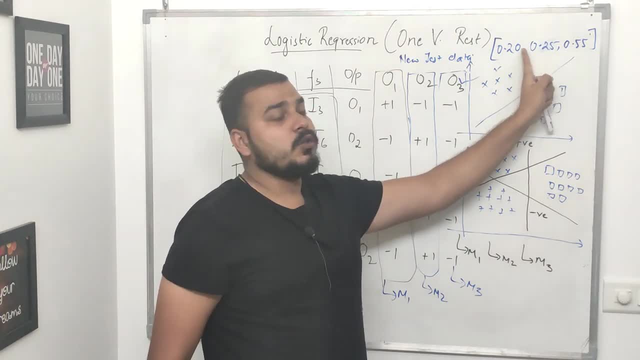 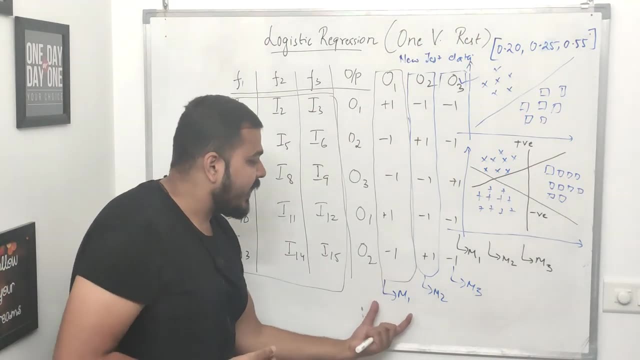 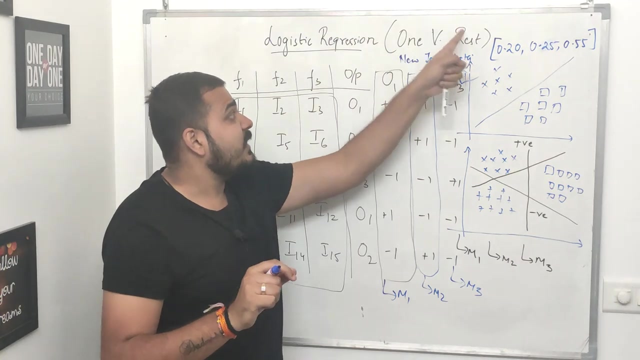 having the highest probability okay, from all this two that we are actually comparing. so this is how one versus rest is actually implemented independently. we'll be creating m1, m2, m3 model and we are not doing it internally. the logistic regression is working on that and for that, to set this particular parameter, there is some parameter called as multi-class. 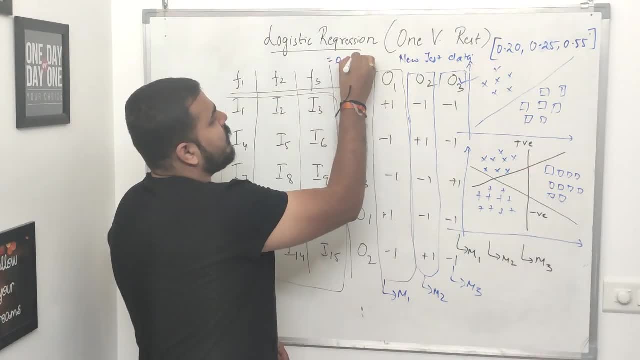 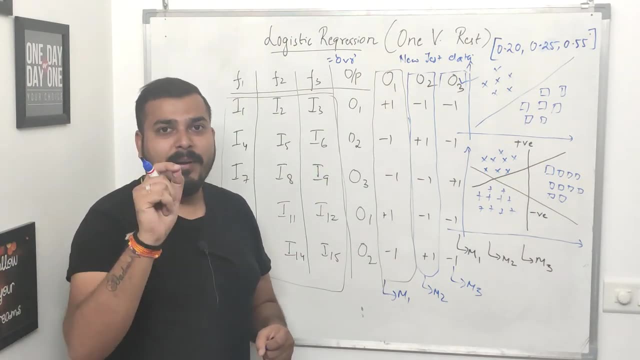 and there you have to set it as ovr. okay, when you are doing the coding mechanism. it is pretty much simple. i'll also give you a link where you can see that how it is actually implemented. there is just one parameter called as multi-class. we have to set it as ovr, automatically, it will treat.